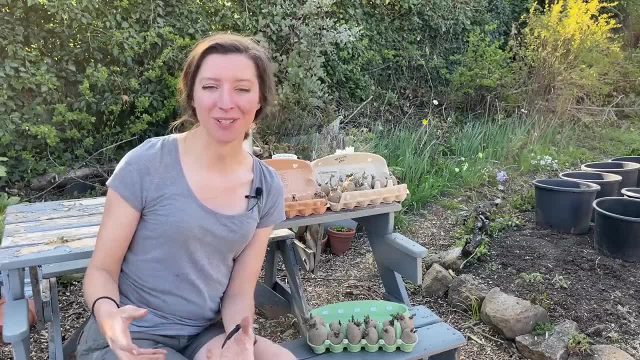 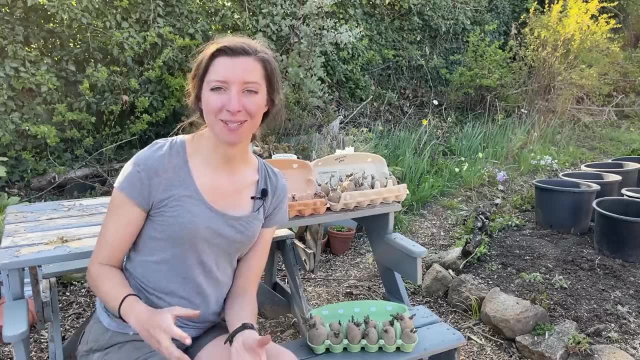 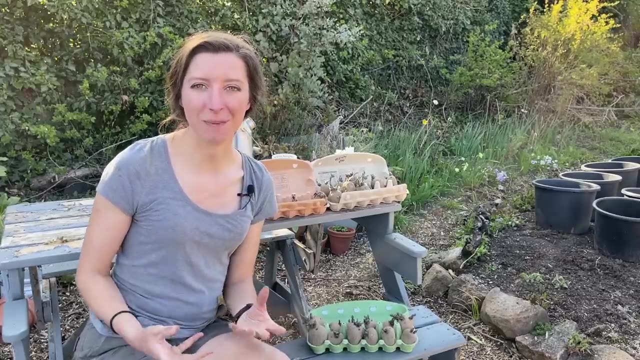 ready for you. You don't have stray potatoes that get lost in your soil and then grow back again with the hard work of digging them out of the soil. you're not going to be disturbing the soil, so it's great for no dig. You're also not going to be slicing through any potatoes with your fork or 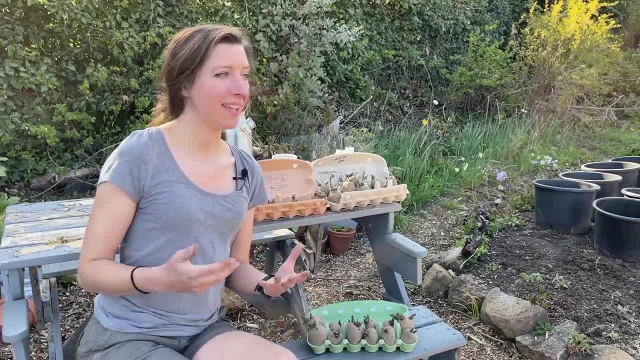 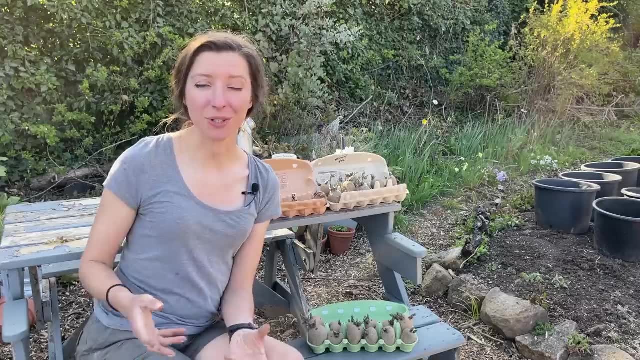 a spade when you're harvesting them because, again, you just tip them out. If it's in a pot, you can move it. so if it starts to get too wet, too dry, if you're worried about the frost, you know you can move your pot to a different location. they're not in the ground permanently, But some of the 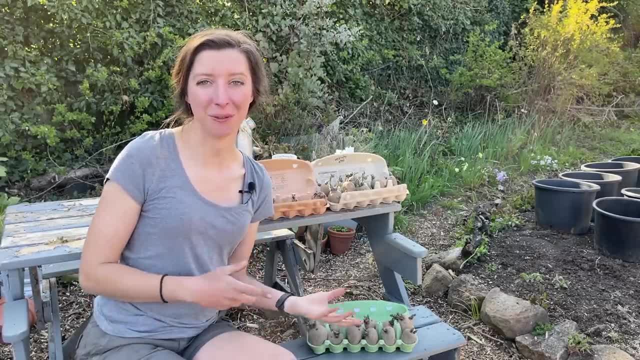 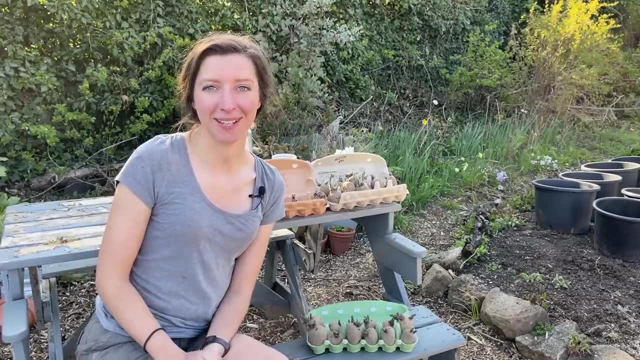 drawbacks are it does involve compost. you need to buy compost to fill the pot And they can be a little bit heavy to move. but really there aren't that many drawbacks to growing in containers and it's just how I grow them now. So I've got here my potatoes that I've already. 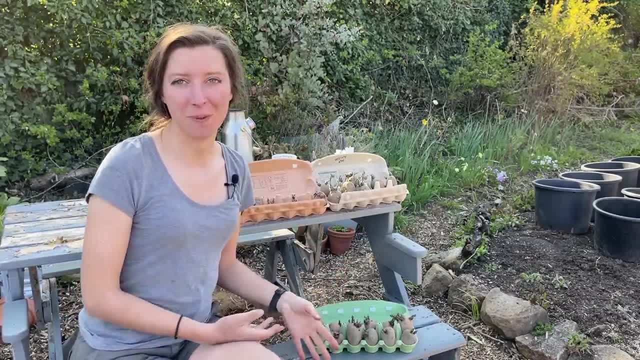 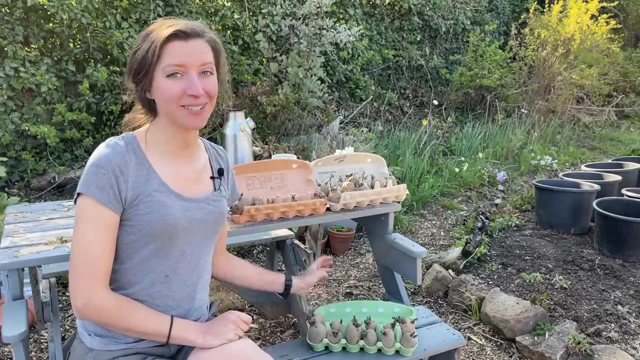 chitted. We've got quite a few varieties this year and I will have some spare that I'll give to friends and neighbours, anybody that wants them. But some of the varieties I have here are King Edward and Cara, so they're our main crops- good old rounders for chipping, mashing, baking. 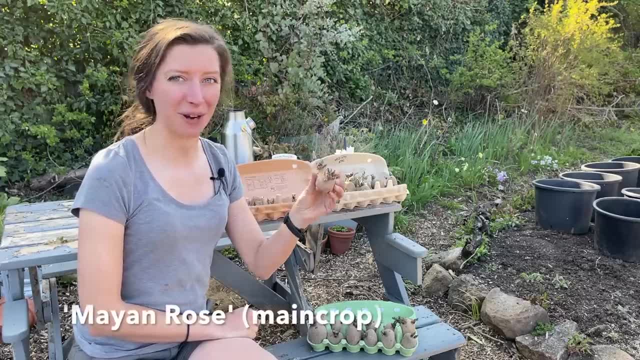 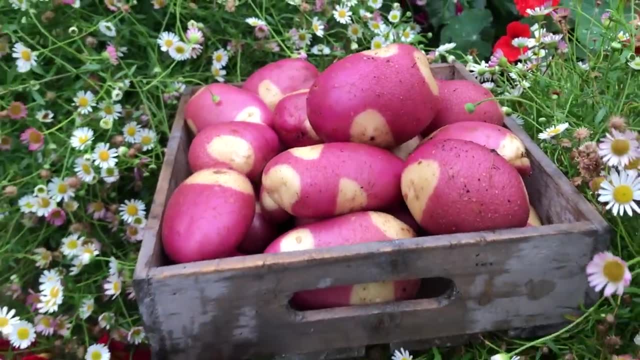 that kind of thing. This one here is the Mayan Rose. I did get hold of Pink Gypsy, which is my usual choice, the one with the white flesh with pink spots on the outside. This one looks very similar and will hopefully taste quite similar too, because 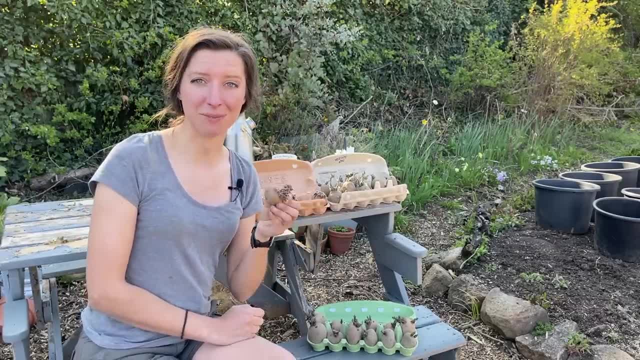 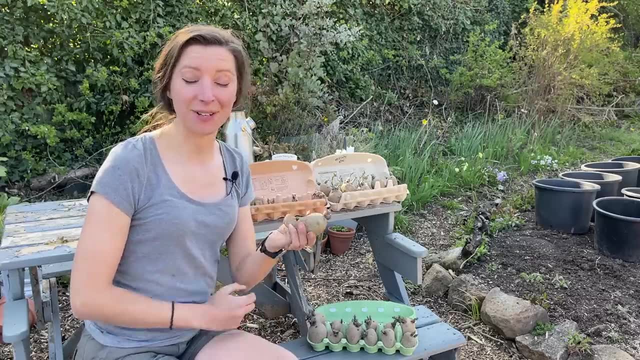 I really do like that one. But yeah, Mayan Rose is my alternative to Pink Gypsy this year. My favourite second early is Charlotte, because they grow so well for me here and you can harvest them as small new potatoes or let them grow on a bit to get a bit bigger, and you know Charlotte's. 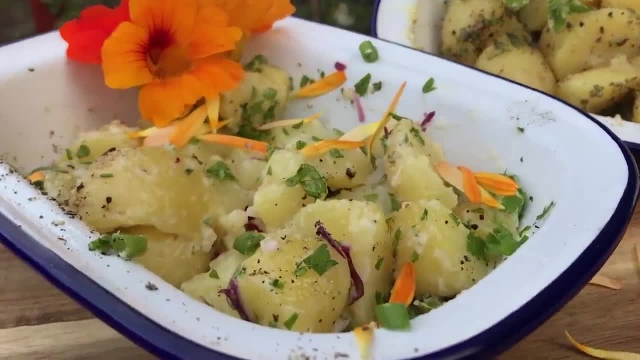 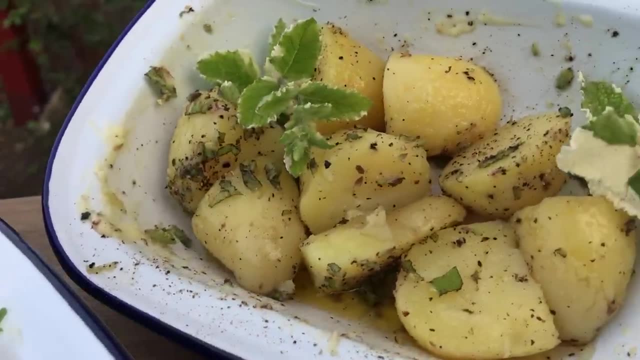 just a really good favourite for a lot of people And I just love them, you know, slowly steamed, covered in butter, maybe a bit of mint sauce, just so good, one of my favourites. I've also got a first early which I could have planted in March. 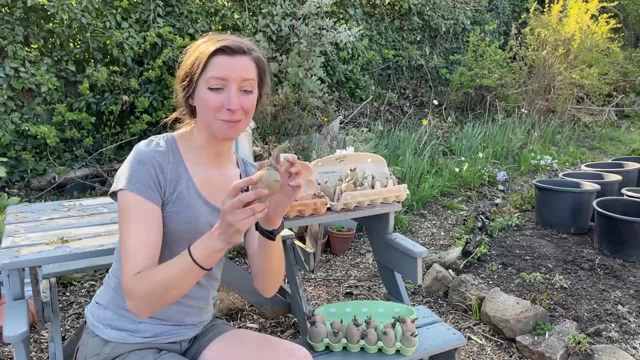 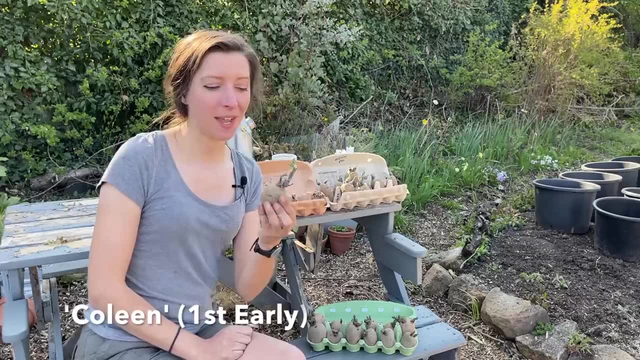 to get a really early crop. You can see it's growing much bigger than all the others already because it's a fast growing crop. This one's called Colleen. I haven't tried it before. I do find that some first earlies don't have as much flavour as the others, like the later croppers. 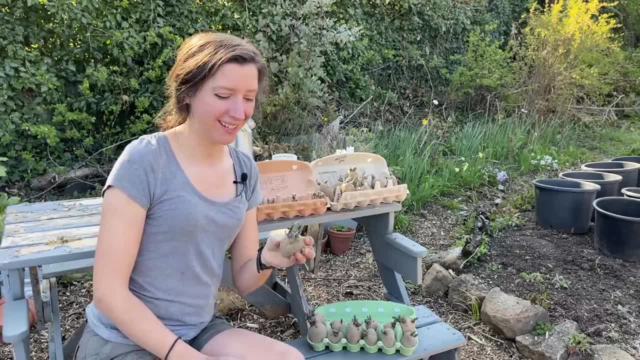 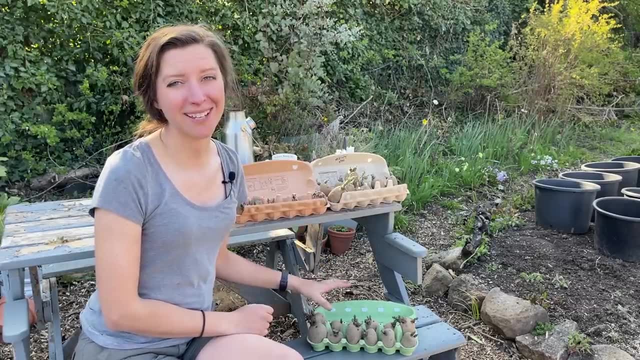 But it's always just good to get something a bit earlier than all the others. So I'll be growing these in smaller containers because they're going to be a lot quicker and smaller potatoes. But yeah, Cara is my absolute favourite main crop. They're the ones that get really big. 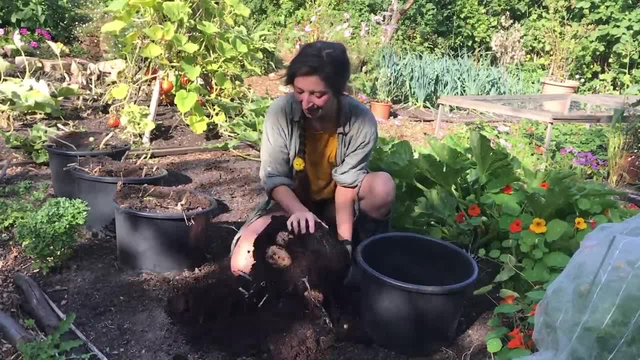 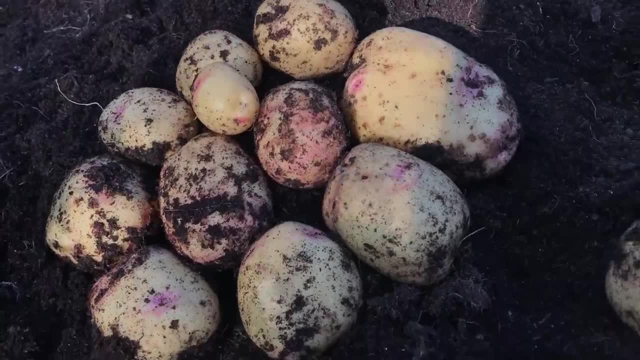 you saw me harvest them last year. I had some great Whoppers from my pots last year- and they just mash well, they bake well, they roast. You can make jacket potatoes, make wedges with them. they're so versatile And I'll kid you not. 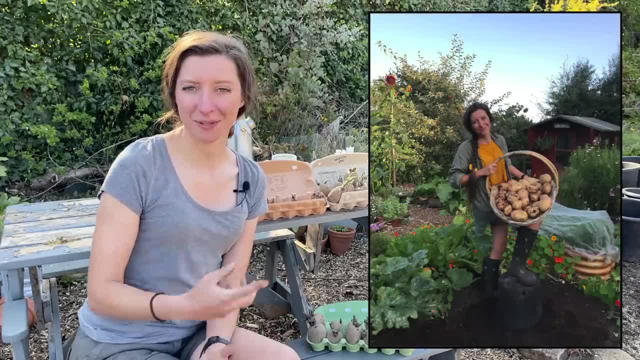 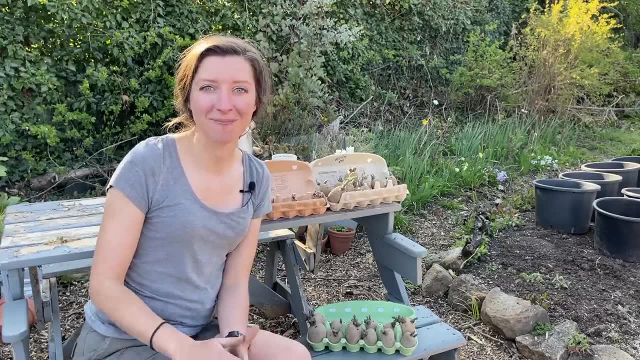 the pots out of my basement to reuse them for my potatoes. it's where I stored them over winter. I still had some in there that were ready to harvest. I didn't realise I'd completely forgotten about them. They did start to regrow a little bit. 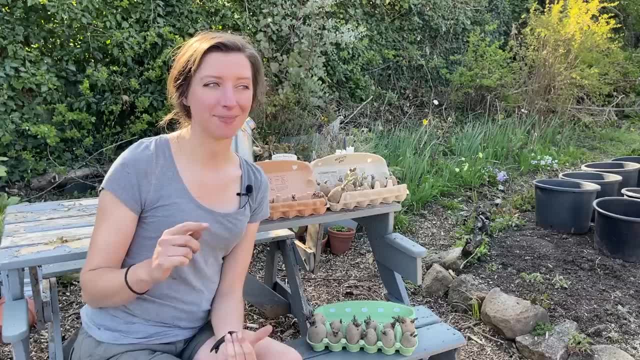 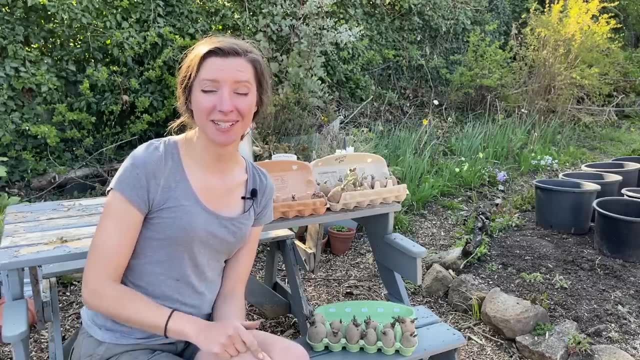 but they're still fresh and edible. So I harvested them mid-September and they're still fresh to eat now, towards the middle of April. So that's over six months in storage and they're still good to eat. So it's worthwhile picking varieties that will suit your style. 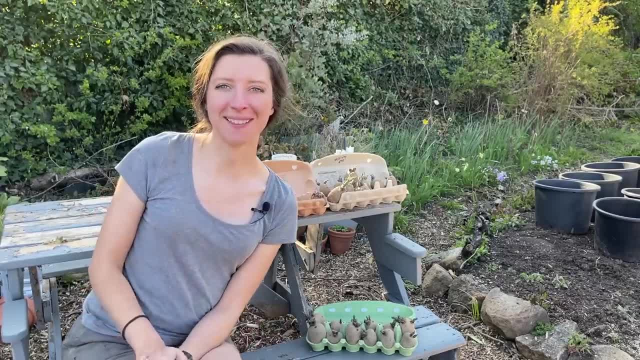 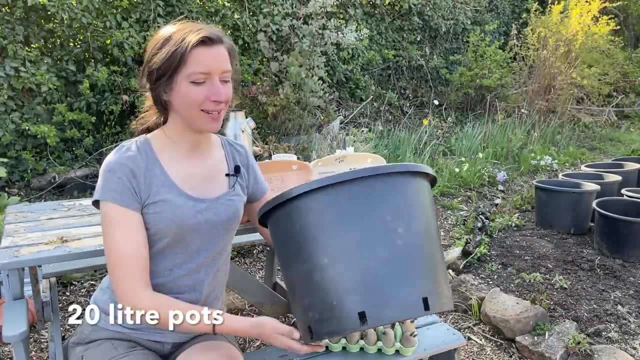 whether you want to store them, eat them straight away. So how do we plant them in containers? Well, I use these rather large 20 litre pots and unless you're buying big trees or shrubs, you won't really be able to get hold of these. But if 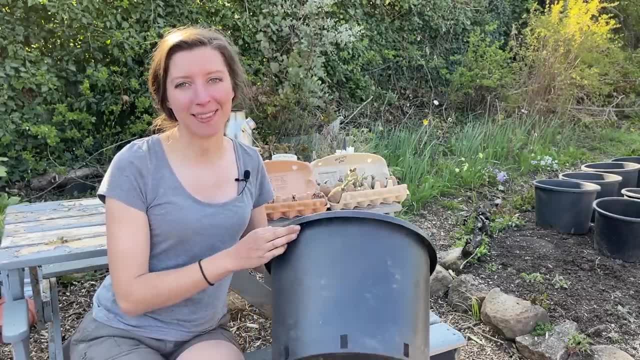 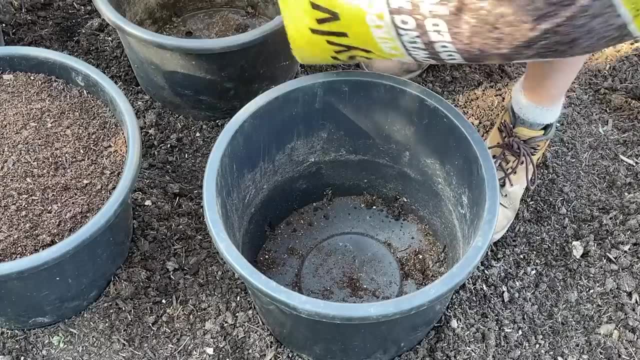 you go to your local garden centre or nursery, they may have some spare that they might be able to give you or you might be able to buy for a small charge. So yeah, I grow all of these in 20 litre containers. First of all, I put a small layer of compost in the bottom. 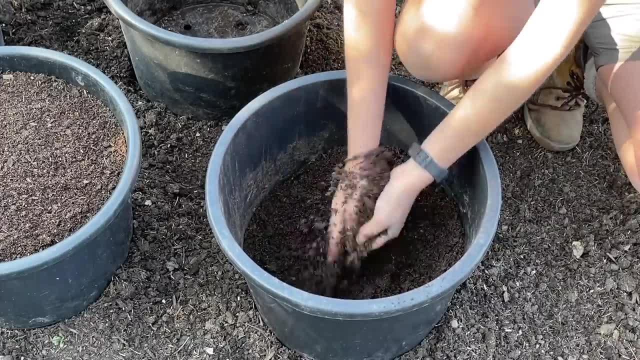 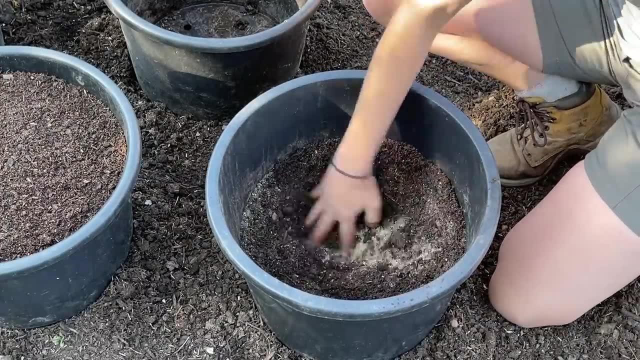 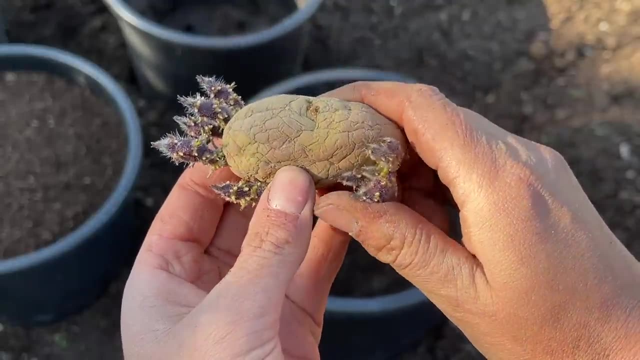 using a peat-free compost, And in the bottom layer I also mix in a scoop of bloodfish and bone- And this is the sort of fertiliser that I use for my potatoes- And I just mix it into that bottom layer. I then take the potato and if it has three or more shoots, I rub them off. So 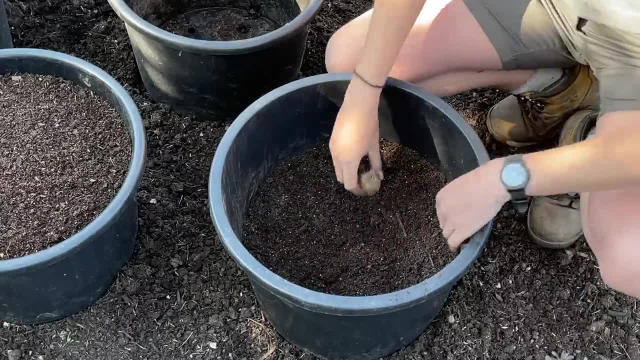 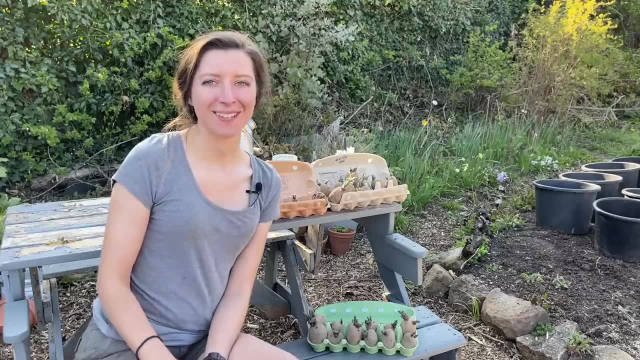 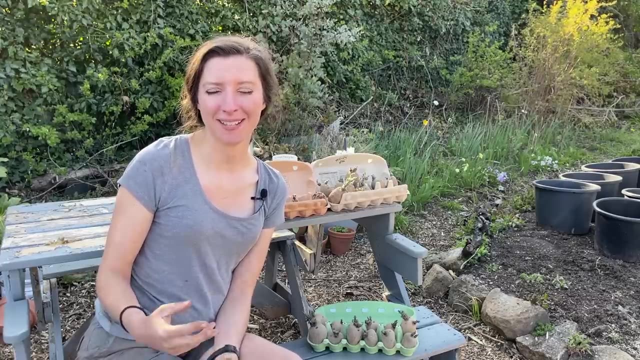 I only really want three chits per potato, And then I plant it in the pot in the middle, with it going upwards. So how many potatoes should you put in a pot? Well, that depends on the variety you're growing, whether it's an early, a main crop. If you're growing it as an early, you may. 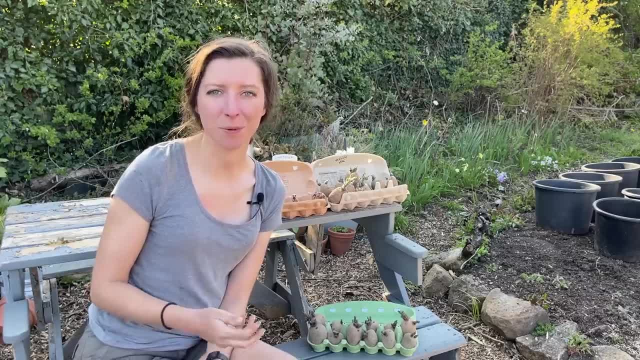 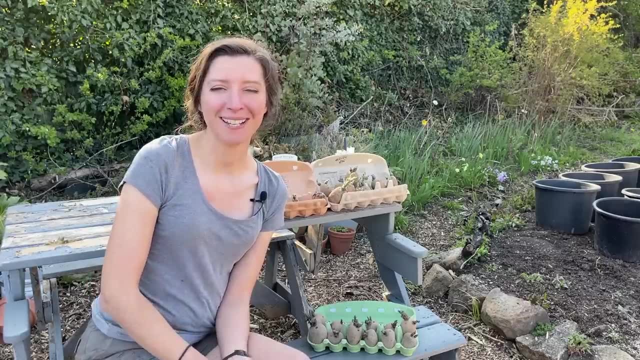 want to put two or three in a pot, It means you'll get smaller potatoes but more of them, Whereas if you just put one per pot, you'll get bigger potatoes but fewer of them. It also depends, obviously, on the pot size. If you're using a very small pot, you might only want to put. 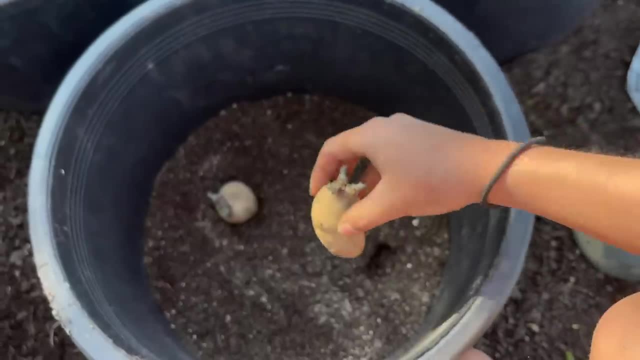 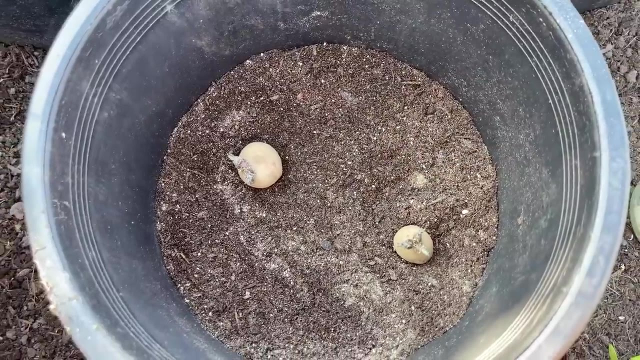 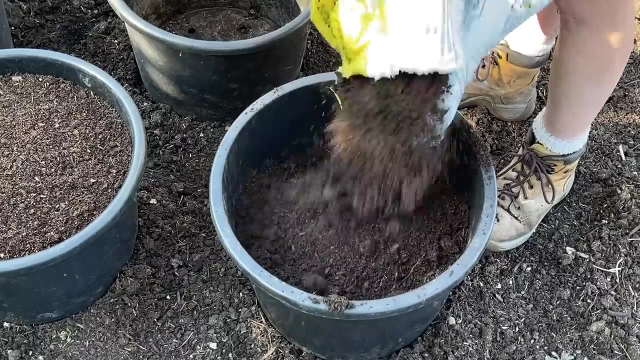 one potato in it. For my first early and second early potatoes I'll put two potatoes per pot, But for my main crops I will only use one potato per 20 litre pot And once the potato is in it's just a case of topping up the rest of the container with compost. I do it right to the top. 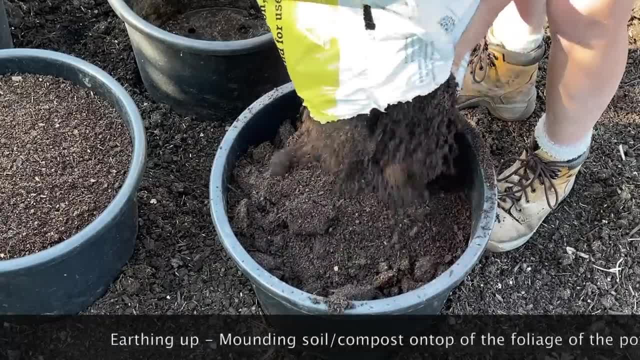 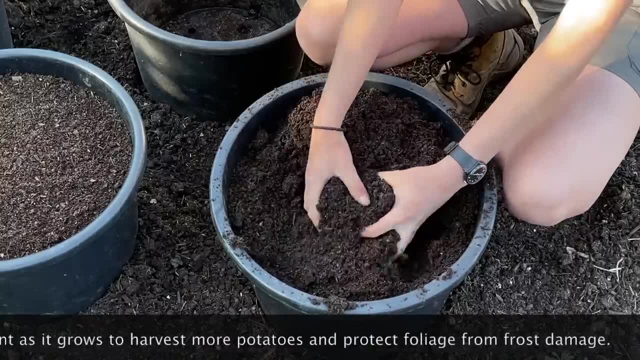 I don't faff about with earthing up in containers because I find that they grow so fast. I don't in the past only had time to earth them up once Before they sort of reach the top of the pot anyway, So I don't waste any time doing that. 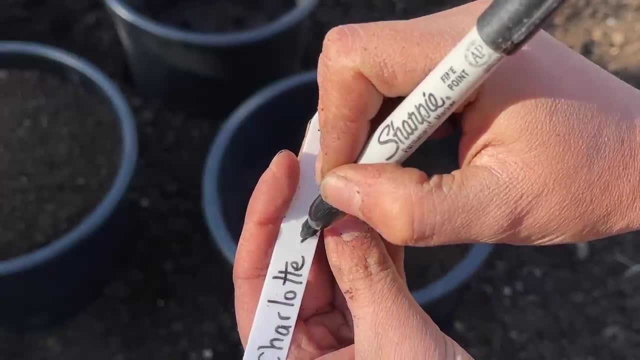 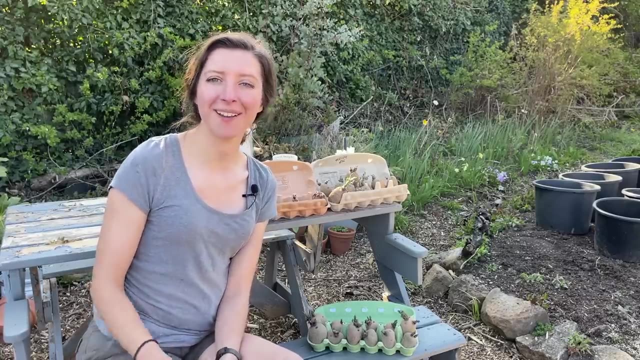 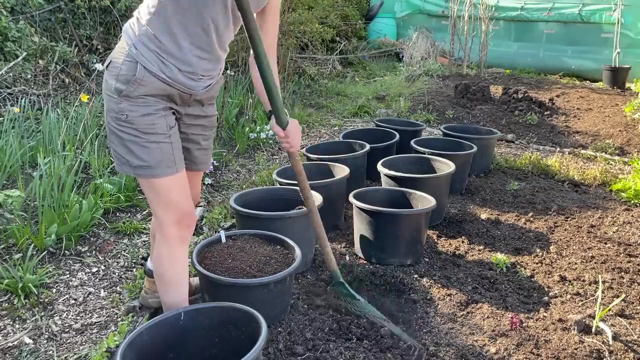 So I fit it right to the top, And then it's just a case of watering it in. On the patch of soil where I'm growing my containers, I actually rake the earth a little bit so that I can bury the pot into the soil by an inch or two, And that means that the holes of the container are covered by. 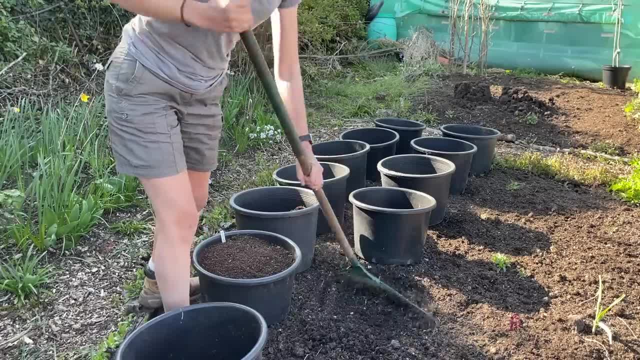 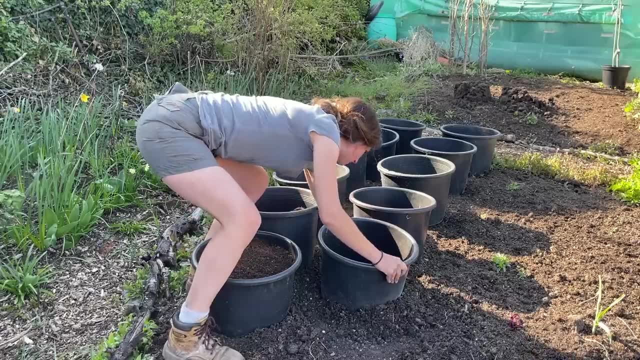 compost, So they're not going to dry out as much. And also it means that if the roots grow on and through those pockets, those holes, they can actually reach down further into the soil to get some more moisture. When you're growing your potatoes in containers, it's really important that. 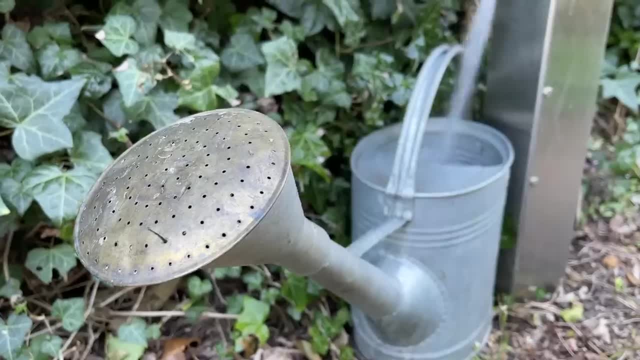 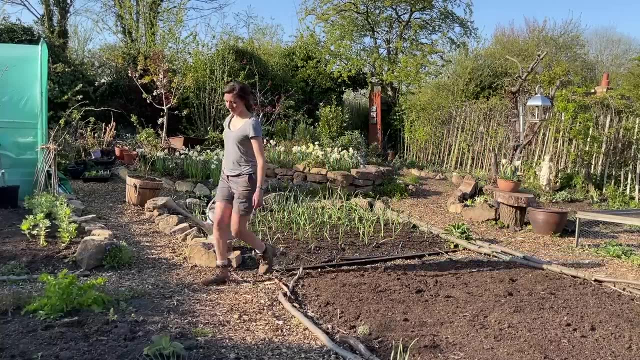 they don't dry out. Potatoes do like it quite damp, So I try not to let the soil in the pots dry out, And it can be quite tricky to keep on top of that in the summer months or if we have a particularly hot and dry spring. So make sure that you're keeping your pots well watered.